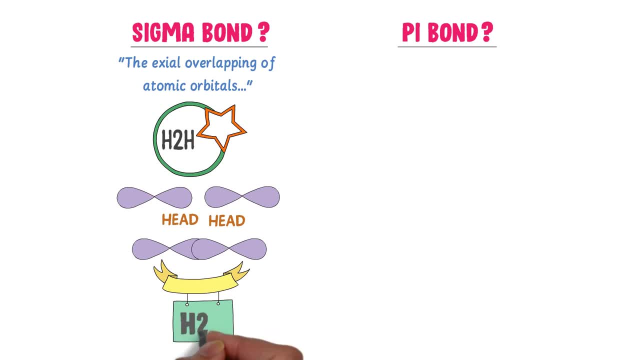 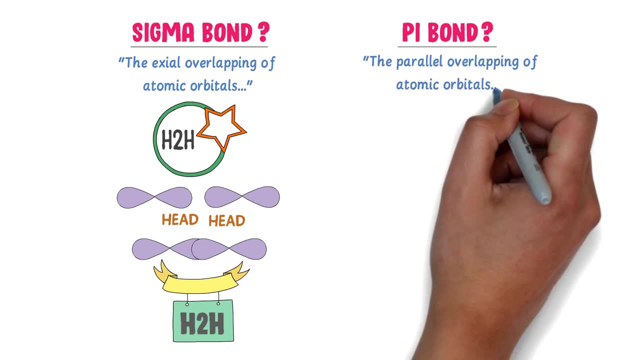 When they both overlap headwise, it is called head to head overlapping. As a result, they form sigma bond, While the parallel overlapping of atomic orbitals always form pi bond. Parallel overlapping of atomic orbital is also known as side to side overlapping. 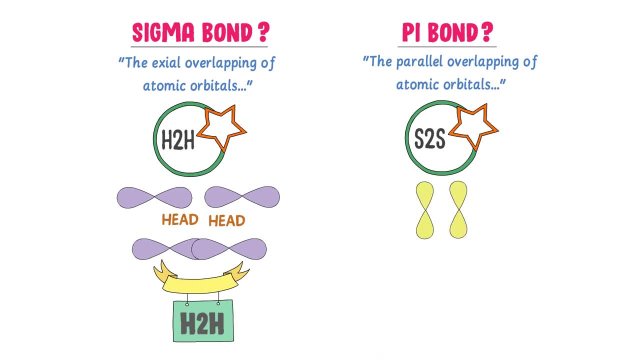 For example, consider these two p orbitals. This is the side of this p orbital and this is the side of this p orbital When they overlap sidewise, it is called as side to side overlapping. Just note it down that head to head overlapping of atomic orbitals always generate sigma bond. 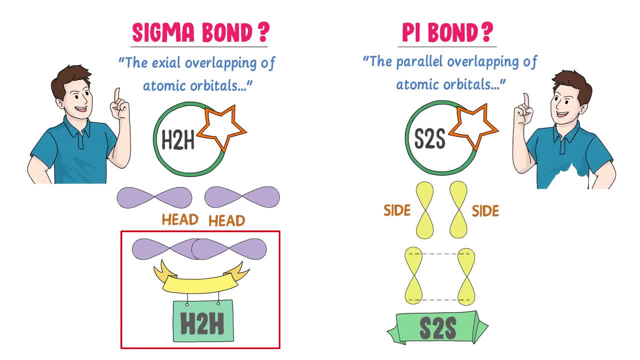 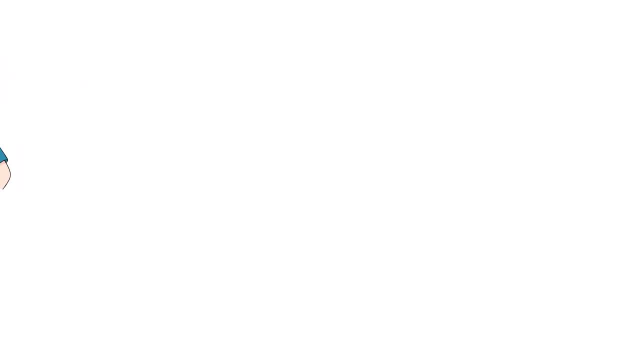 Like in this example, While side to side overlapping of atomic orbitals always generate pi bond, Like in this example. Now, what are the possible combinations of atomic orbitals that form sigma bond and pi bond? Well, we know that head to head overlapping of atomic orbitals always form sigma bond. 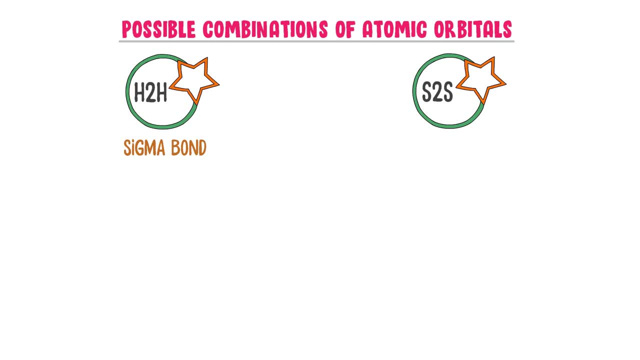 And side to side overlapping of atomic orbitals always form pi bond. For example, s orbital plus s orbital always overlap headwise to form sigma bond. Secondly, s orbital and p orbital always overlap headwise to form sigma bond In case of p-p overlapping. 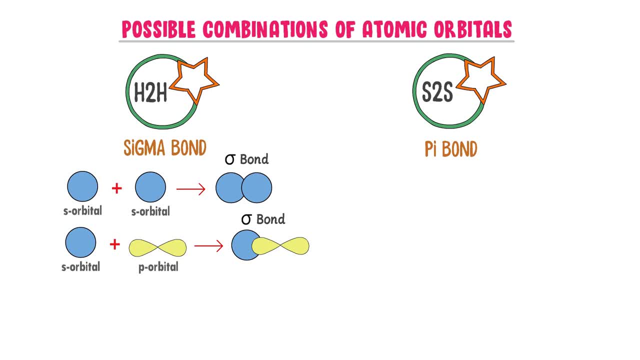 it may either form sigma bond or pi bond, depending upon its overlapping. For instance, if p orbital overlap headwise, it will form sigma bond. If p orbitals overlap sidewise, they will form pi bond. Thus, only sidewise overlapping of p orbitals form pi bond. 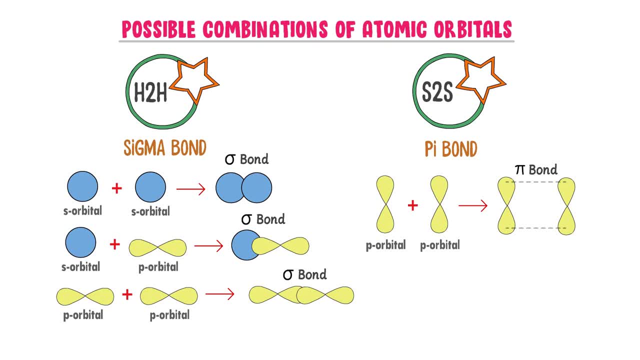 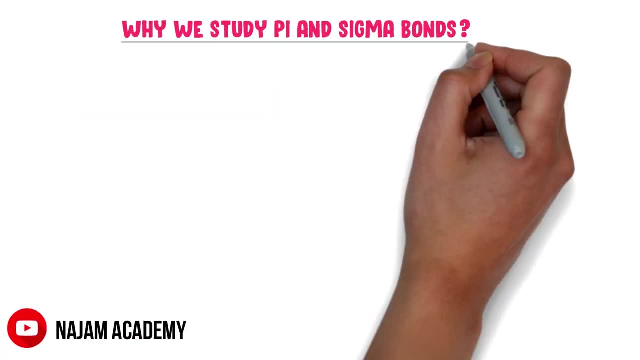 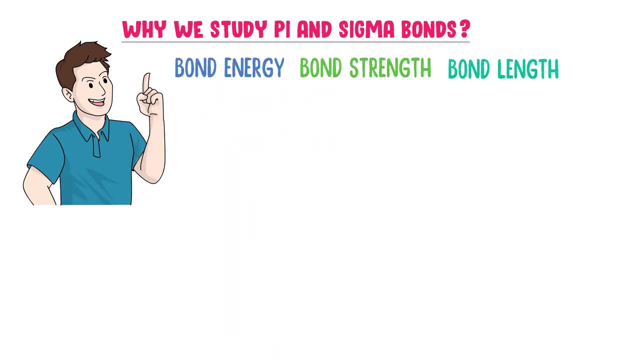 While headwise overlapping of ss, sp, pp orbitals form sigma bonds. Also, you should learn that why we study sigma and pi bonds. Well, sigma and pi bonds explain the bond energy, bond strength and bond length of a molecule. For example, consider sigma bond between these two p orbitals. 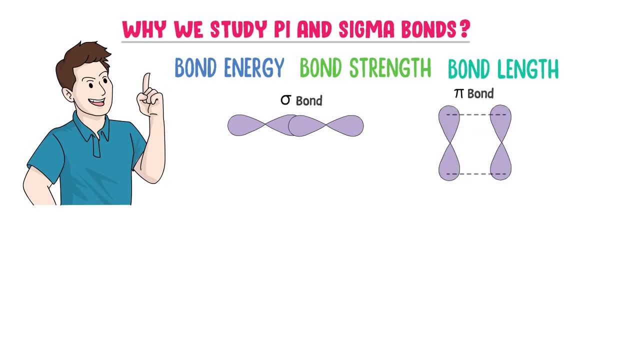 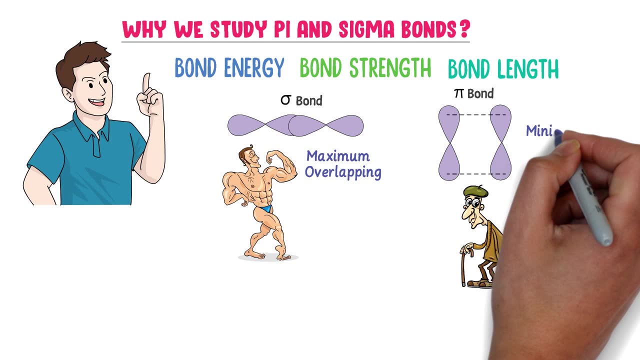 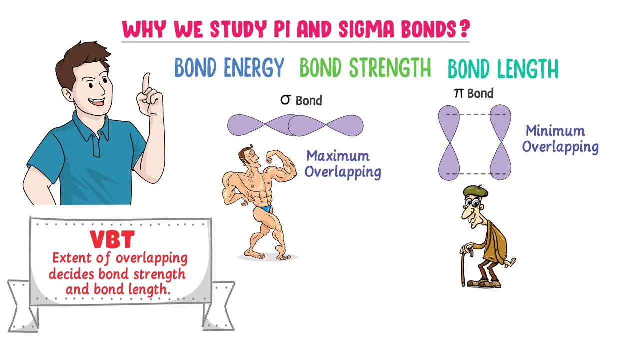 and pi bond between these two p orbitals. Remember that there is always maximum overlapping taking place in sigma bond, While there is always minimum overlapping taking place in pi bond. Also, according to valence bond theory, extent of degree of overlapping decides the bond strength, bond energy and bond length. So we therefore say that sigma bond is stronger. 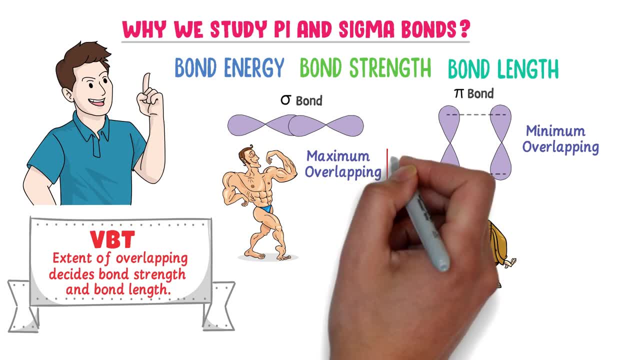 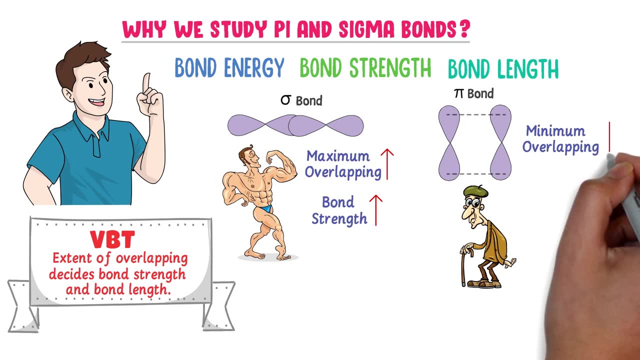 than pi bond. Secondly, the maximum the overlapping between two orbitals, the greater will be the bond strength or bond energy, While minimum the overlapping between two orbitals, the smaller will be the bond strength or bond energy. Also, let me teach you the bond strength, bond energy. 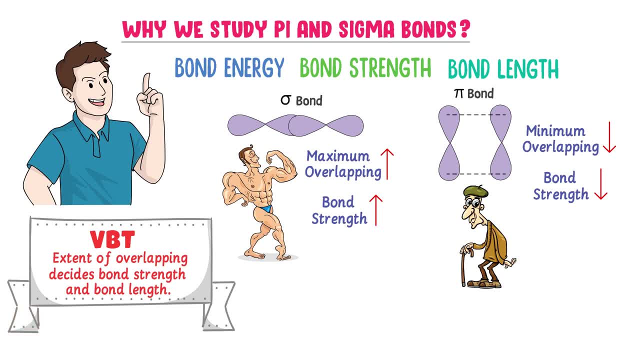 and different combinations of atomic orbitals. For example, an head-to-head overlapping of two pi orbitals or sigma bond between two orbitals. there is maximum overlapping, So it forms strongest bond or it has high bond strength or high bond energy. Secondly, the sigma bond of sp. 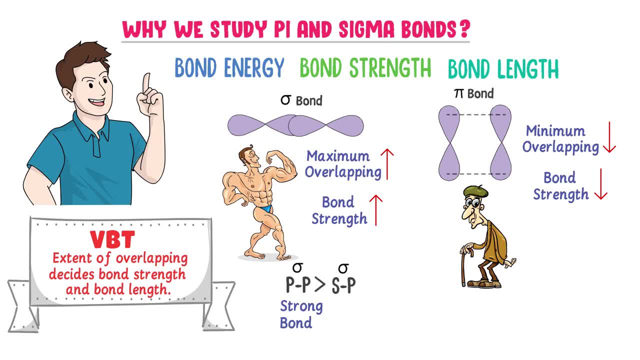 orbital also have greater bond energy, but lesser than pp overlapping. Thirdly, the sigma bond of ss orbital has lesser bond energy than sp overlapping. And finally, the pi bond of pp orbital has smallest bond energy because the extent of overlapping between them is smaller. Now 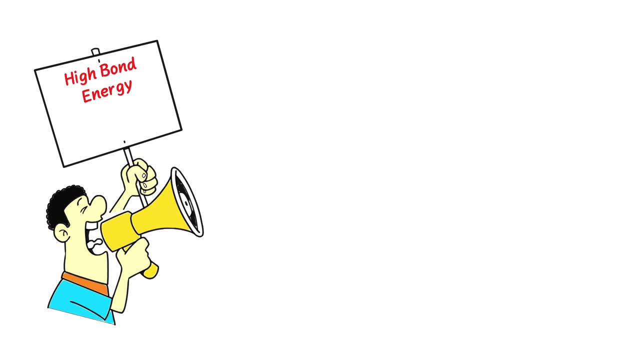 remember that the higher the bond energy or the bond strength, the smaller will be the bond length. For example, in case of sigma bond of ráp orbital, there is high wrong forcing, Hence both the orbitals are close to each and the bond length is smaller, while in the case 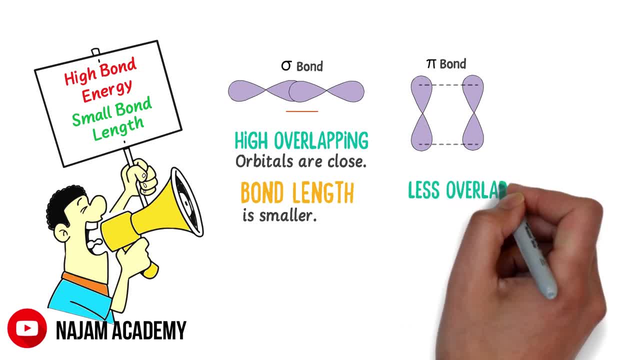 of pi bond ofap orbitals. both the p or aparece이랑, and both the p or are away than each other and the bond length is greater. So this is the order of bond energy Here. let me teach you one bonus MCQs: which bond has more bond energy than what sacb? 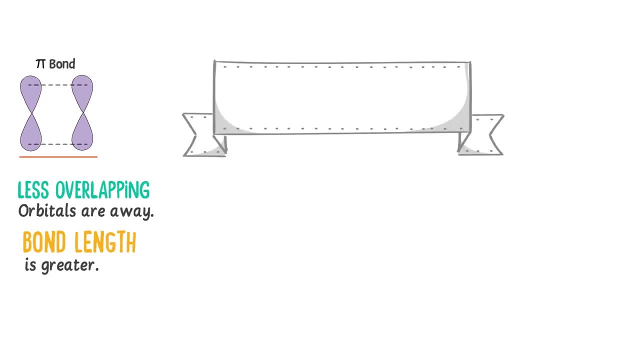 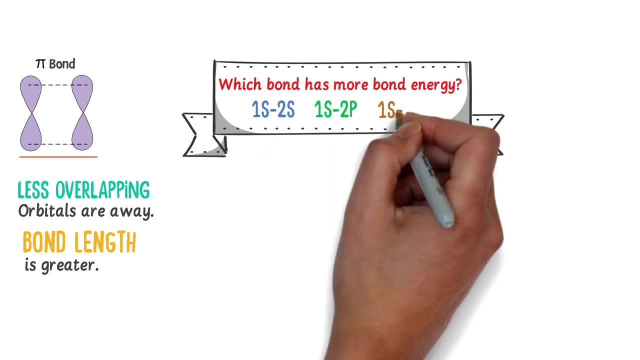 So this is the order of the bond energy. Here let me teach you one bonus MCQs. which bond has more bond energy than other acting bonds, For example, called the sigma And ogni p? in the case of sigma, bond of, are bond strength 1s2s, 1s2p and 1s3s? Well, the answer is 1s2s, Because 1s and 2s are. 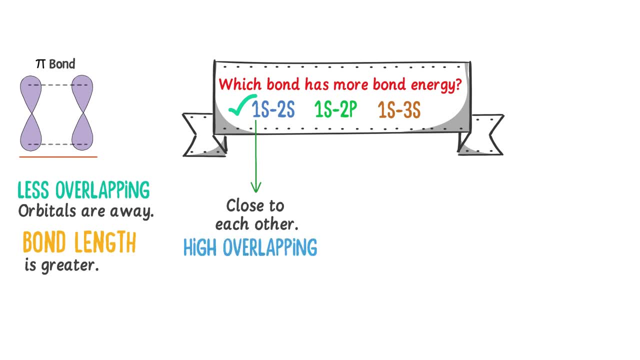 close to each other, so the extent of overlapping between them will be maximum and they will form strong bond. But its bond length will be minimum While 1s3s are away from each other, so the extent of overlapping will be minimum and its bond energy will be smaller. 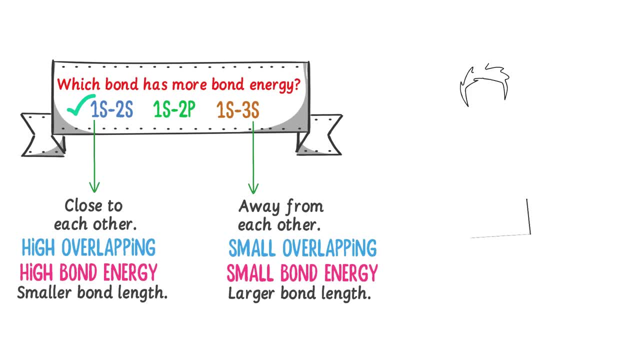 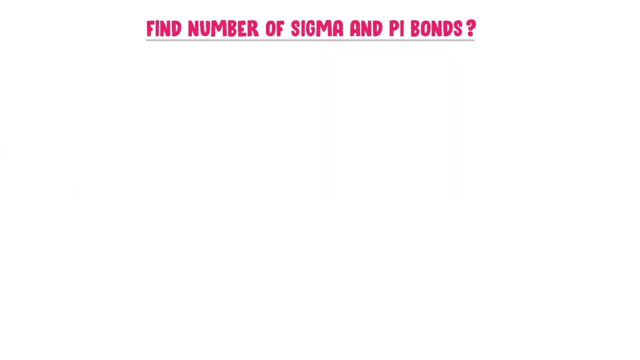 but its bond length will be greater. Therefore, we study sigma and pi bonds because they teach us about bond strength, bond energy and bond length of any molecule. Finally, let me teach you that how you find the number of sigma and pi bonds in a molecule. 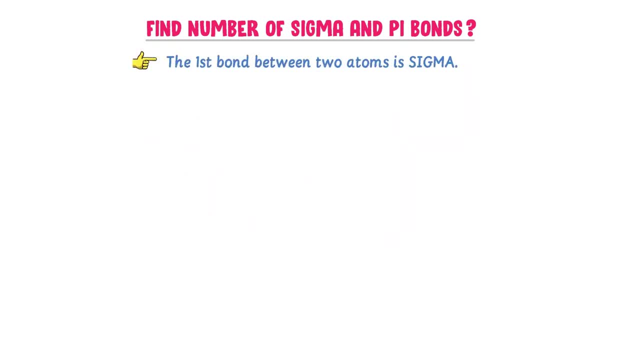 Remember that the first bond between any two atoms will be sigma. It is impossible that the first bond between any two atoms would be pi. The second and third bonds between them will be pi. For example, find the number of sigma and pi bonds in water. 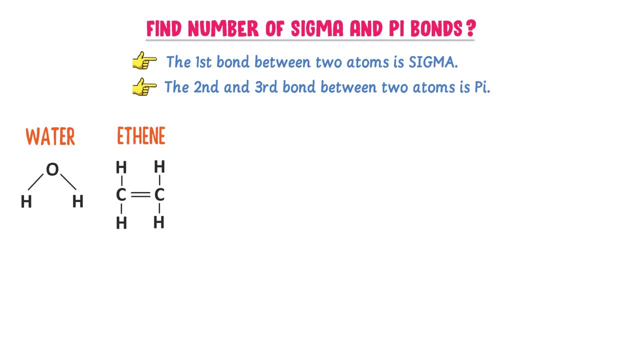 H2O, ethene, C2H4,, ethane, C2H2,, propionic acid, C3H5OH and sulfur trioxide, SO3.. Well, in case of water, oxygen forms single bond with this hydrogen, So it is sigma bond. Oxygen also forms single bond with this hydrogen. 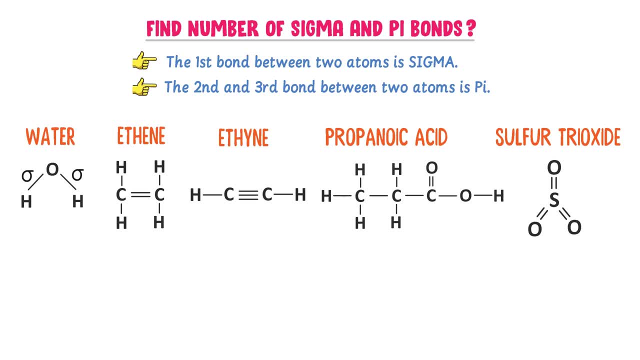 atom, So it is also sigma bond. Thus, there are two sigma bonds present in water, While there is no pi bond present in water. In case of ethene, carbon forms sigma bond with this hydrogen atom. Carbon forms sigma bond with this hydrogen atom. 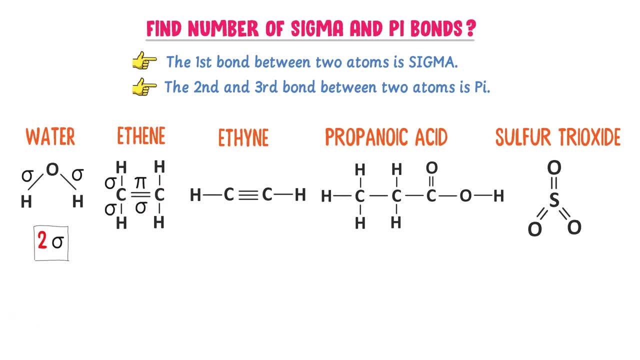 The first bond between carbon and carbon is sigma bond. The second bond between carbon and carbon is pi bond. This is also sigma bond. This is also sigma bond. So there are five sigma bonds and one pi bond present in ethane. In case of ethane, this: 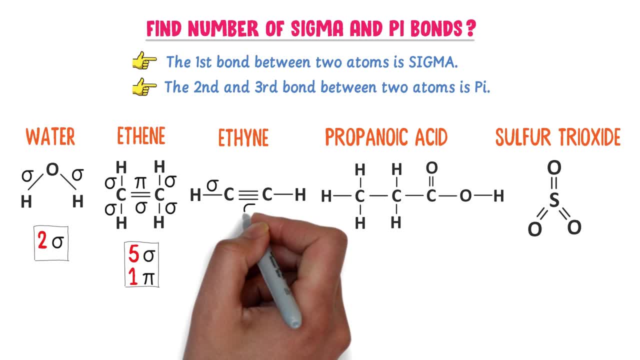 is sigma bond. The first carbon-carbon bond is sigma. The second bond between carbon-carbon is pi. The third is also pi And this is also sigma bond. So there are three sigma bonds and two pi bonds present in ethane. 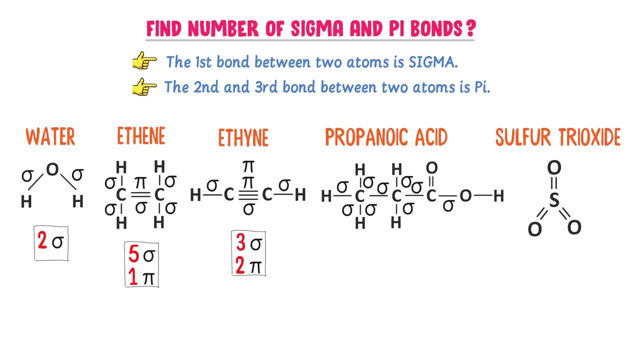 In case of propanoic acid, all the single bonds are sigma bonds, while the first bond between carbon and oxygen is sigma and the second bond is pi. So there are ten sigma bonds and one pi bonds present in propanoic acid.